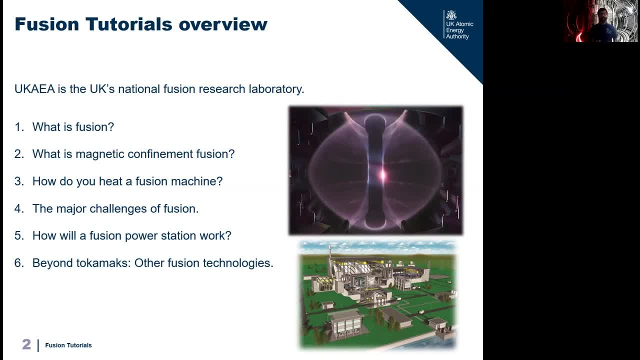 in fusion and some of the work that we are doing at UKAA and around the world to try and overcome those challenges. Then, as we get towards the end of this series, we will have a little recap and a look at all of the things that you have learnt so far and how. 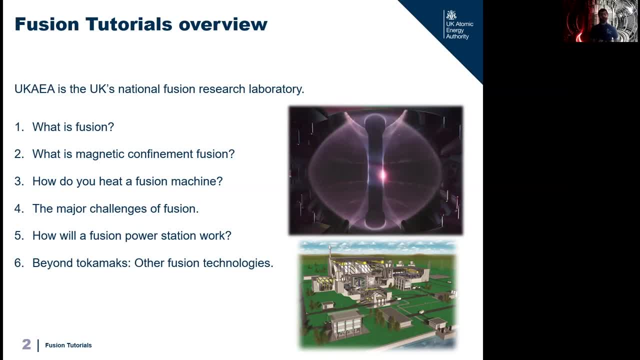 they all need to come together to produce fusion power. We will also be looking at how we can produce a fusion power station. We will finish off the series looking at lots of other ways of producing fusion and other technologies beyond tokamak, which is the main fusion energy device that we are researching here in the UK. 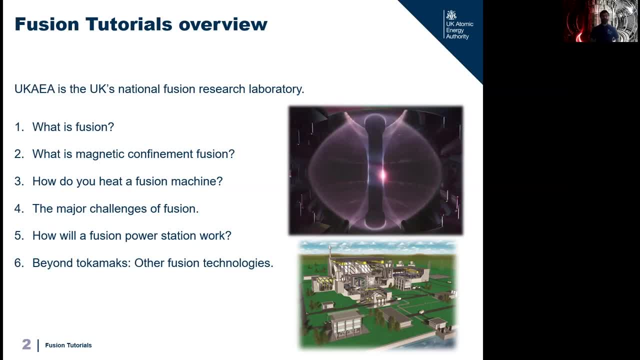 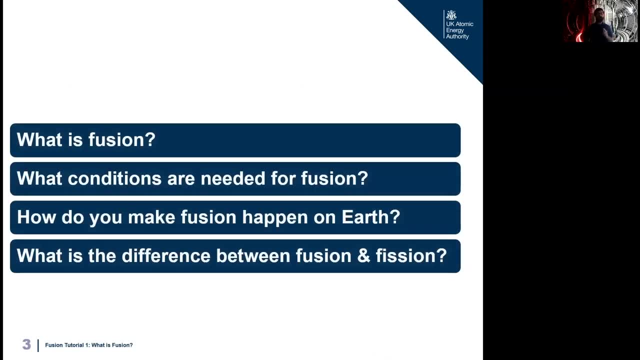 So we will jump right into our first tutorial. In this one, I want to start with being able to ask some questions. I am going to use my favourite topic at this time, The topic that answer four questions. Firstly, we will just look at what is fusion and find ourselves a very simple 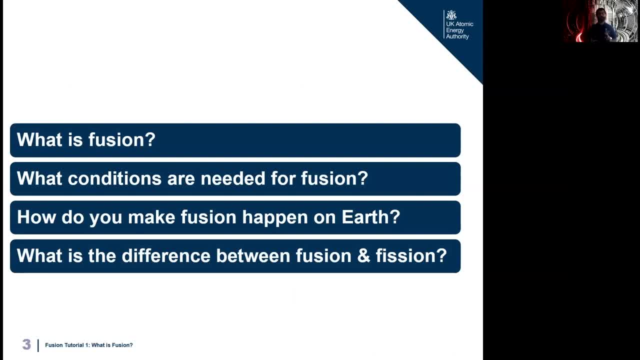 definition of that. Then we will move on to have a little look at the conditions that are needed to create fusion power And we will move from that to look at how those conditions that might naturally occur in places needs to be modified to make fusion energy here on earth in a form that we 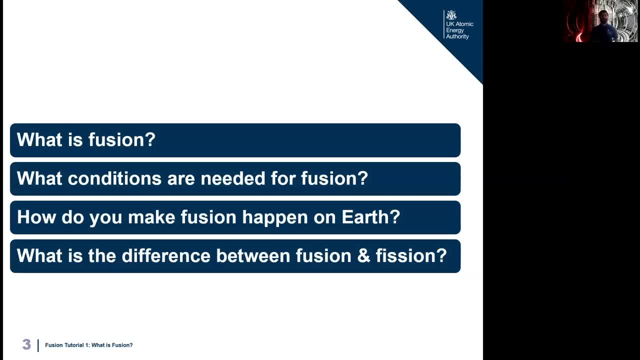 can use to one day power our own homes. And we will, lastly, have a look at the difference between fusion and fission, with fission being a current energy source that we have here on earth that is related in a way to fusion. So what is fusion? 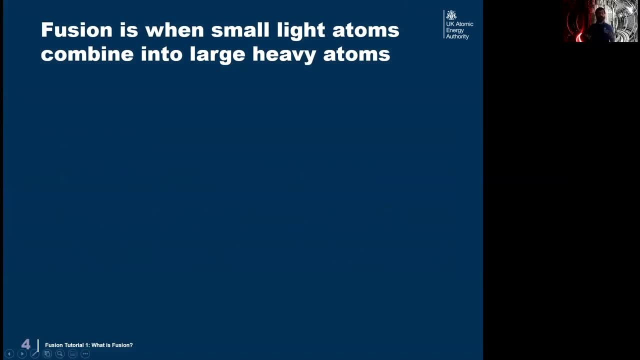 Well, very simply, fusion is when small light atoms come together to form larger, heavier atoms. So if we have a little, look very simply, we have got two atoms here. They need to combine together or fuse. When we do that they produce a larger atom. It is also much heavier than what. 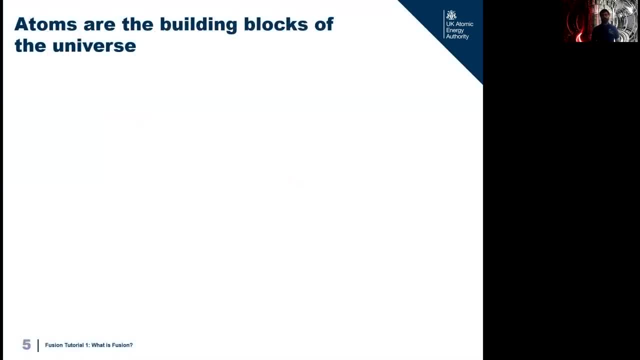 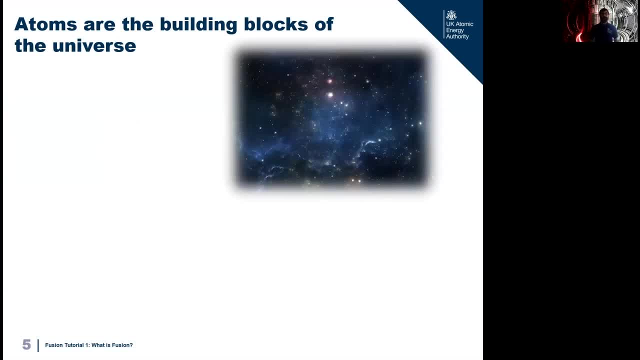 the universe. Well, atoms are just the base of the universe. Well, atoms are just the base of the building blocks of the universe. They make up all the stars and all the planets that are out there. They make up all the gas in the air around us that we breathe. They make up everything in our food. 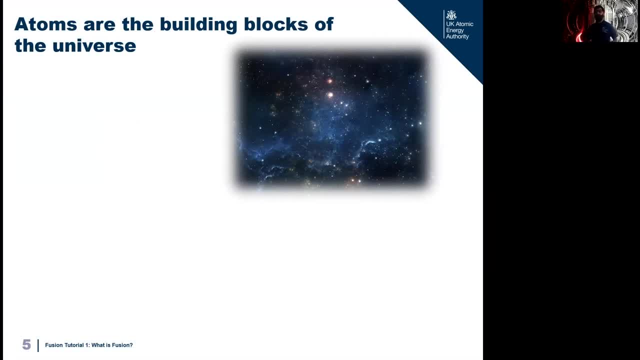 They even well, they make up all of us. They make up plants, They make up bacteria. Everything is made up of atoms, And this is a very basic look at what an atom is like In the very centre of the atom. 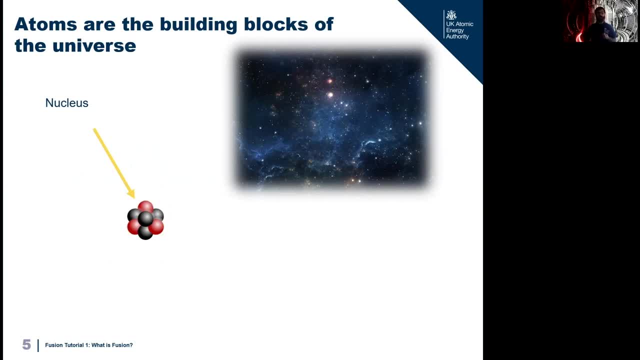 you have a nucleus. Now this is the core of the atom, And when you get lots of them together, you simply just call them nuclei, being the plural of nucleus. Now we're going to have a little closer look at the nucleus itself, because you can see that it's made up of two parts: The nucleus- 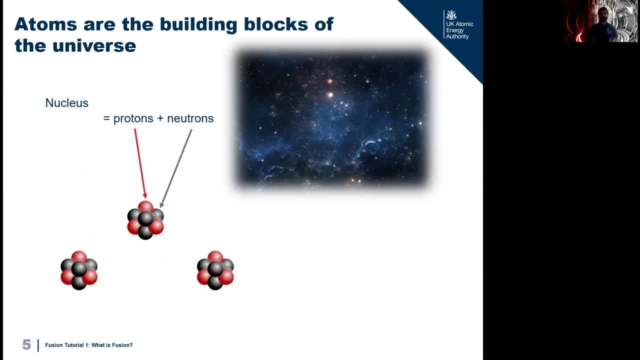 itself is made up of protons and neutrons, And so that's the core of the atom. But there's also things whizzing around the outside of the atom. There's also things whizzing around the outside of the nucleus, And those are electrons. Electrons orbit around the nucleus. 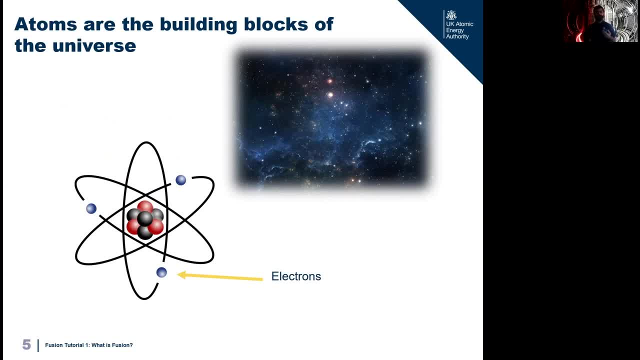 following those black lines to represent the orbits of the electron Now taken together. this is very simply what an atom is. An atom has a core nucleus with protons and neutrons. in And around that nucleus are whizzing electrons, And it's going to be. 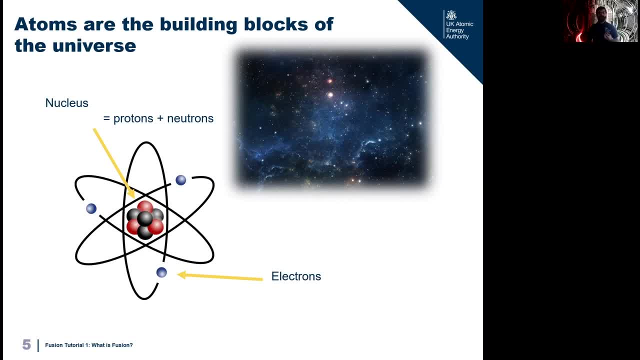 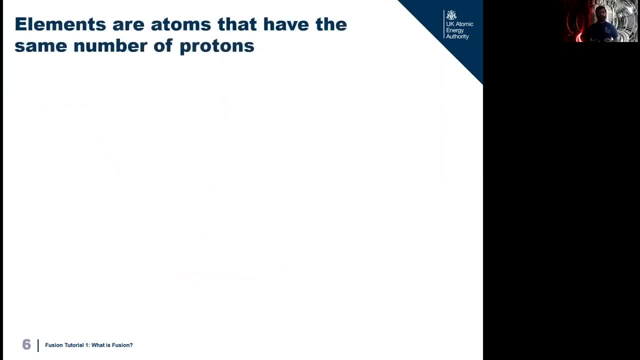 very fundamental to understand these different parts of an atom to help us understand how fusion really works. Now, atoms can be grouped together into elements that share the same properties, And elements are simply atoms that have the same number of protons. So let's just 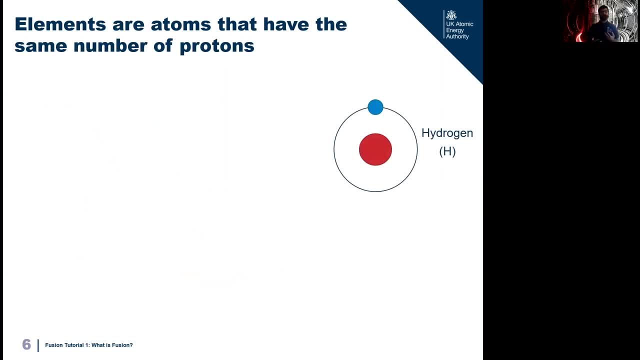 take a look at hydrogen for a moment. Hydrogen is the most basic element out there, And one atom of hydrogen will have one proton in its nucleus- not even any neutrons- and one electron around the outside, And so, no matter what atom of basic hydrogen it might have, we'll always find that it. 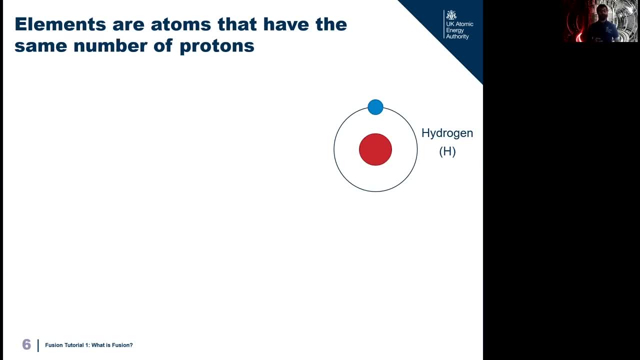 has one proton inside its atom. Now, if we have a little look at helium, helium is the next element that we could find And that is made up of two protons, two neutrons and two electrons. So, even though it can have different numbers of neutrons and electrons, 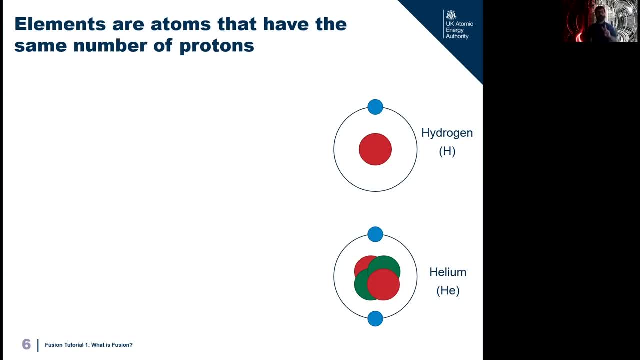 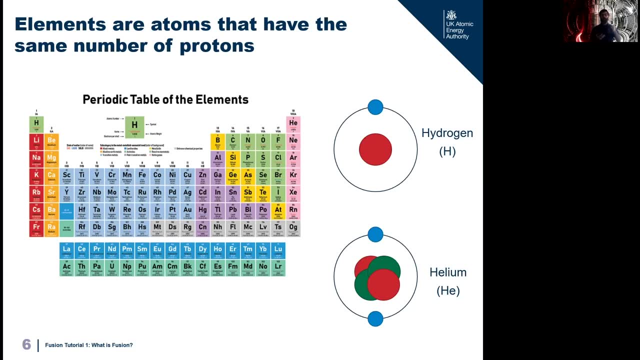 every atom of helium you ever find will have two protons in it, And this goes for any element in the periodic table. No matter which one you pick out, each atom of that element will only have a standard number of protons, And that'll be how you can tell it's an atom of that element. 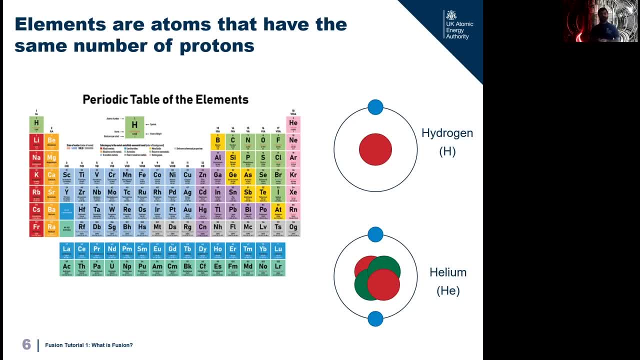 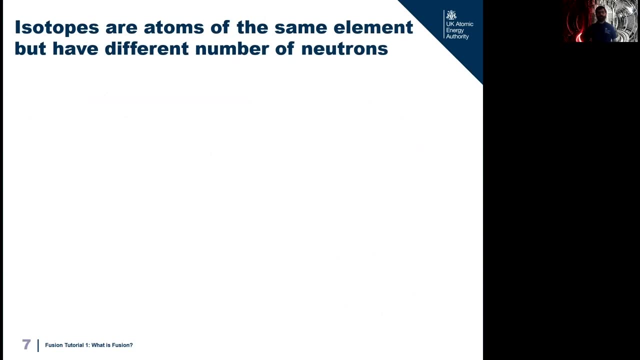 And that all of those elemental atoms will share the same properties. So the properties of a carbon atom will be different to the properties of an oxygen atom based on the number of protons that they have. Now, the next thing I wanted us to look at was isotopes. 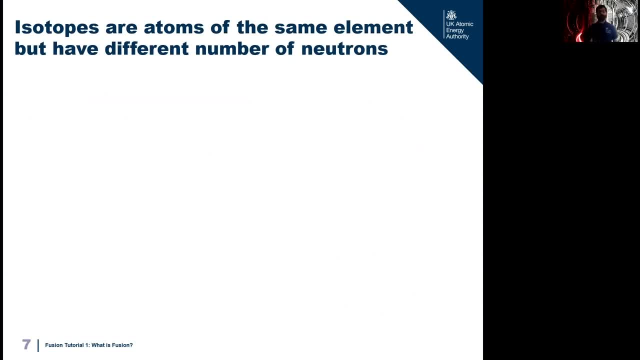 Isotopes are atoms of the same element, but this time they have a different number of neutrons. So again, let's look at hydrogen. Hydrogen, we know it's got one proton, because that's what makes it the element of hydrogen. 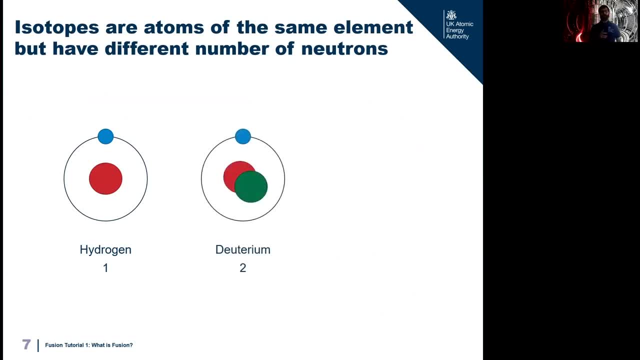 But you can find hydrogen with an extra neutron When we find that we call it deuterium, Or sometimes we call it deuterium, Or sometimes we call it hydrogen too. And deuterium very simply has one proton, one neutron and one electron. 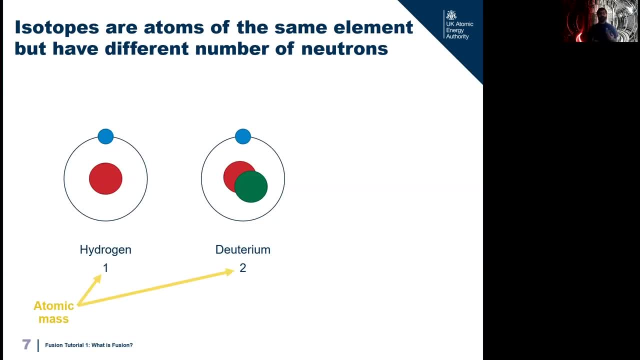 Now the numbers at the bottom are what we call the atomic mass, And they represent how much mass these different isotopes or atoms have. Hydrogen 1 has an atomic mass of 1, because protons have a mass of 1.. 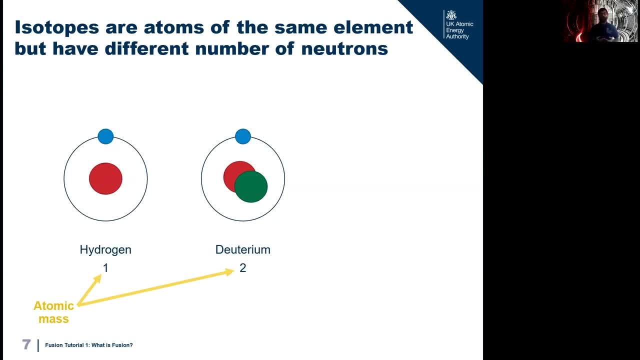 Now, electrons have a mass so small that they're often not included in the atomic mass. The mass of a neutron is also 1.. So with deuterium, when it's got one proton and one neutron, its total atomic mass is 2.. 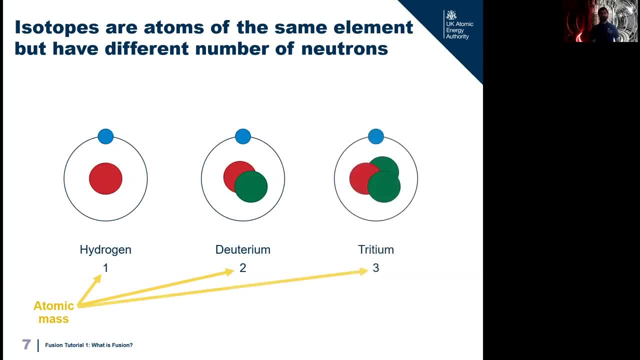 If we look at another isotope, hydrogen tritium, we can see that this one has two neutrons in its nucleus and one proton, And that's what gives it an atomic mass of 3.. Now sometimes we call hydrogen 2, or deuterium, heavy hydrogen, because it's heavier than the basic hydrogen 1.. 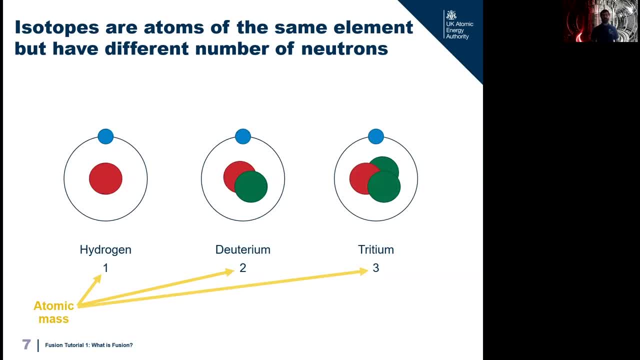 And sometimes we call tritium super heavy hydrogen because it's got even more mass inside the nucleus of a tritium atom. Now, because that could be quite a complicated thing, we just wanted to include another one. We just wanted to include another one. 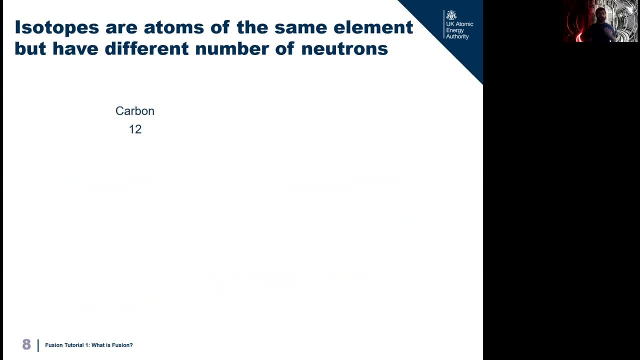 We just wanted to include another example of an isotope. We're going to look at carbon this time. So with carbon, its most common isotope is called carbon 12.. Again, meaning that it has an atomic mass of 12. And the atomic mass is split right in half with carbon 12.. 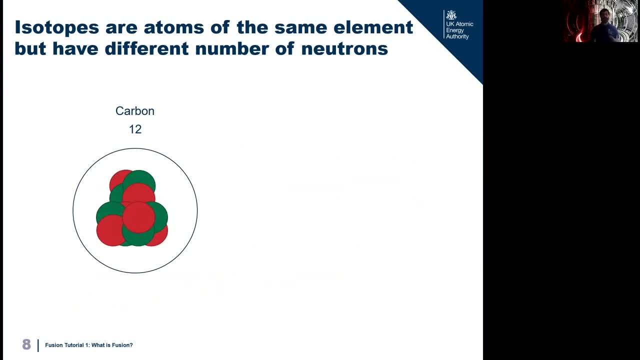 So it's got six protons and six neutrons, giving a total of 12.. However, you can get isotopes of carbon, such as carbon 13. And with this it's just simply got an extra neutron. So this time, seven neutrons, six protons, giving us carbon 13 isotopes. 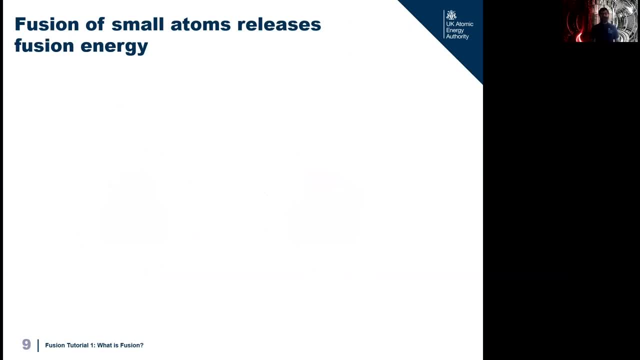 So that's just a very basic look at atoms, elements and isotopes. And fusion is just when any small atoms come together and fuse, releasing fusion energy. Every time fusion of atoms happens, it releases a burst of energy. Now, this is a very, very simple look. 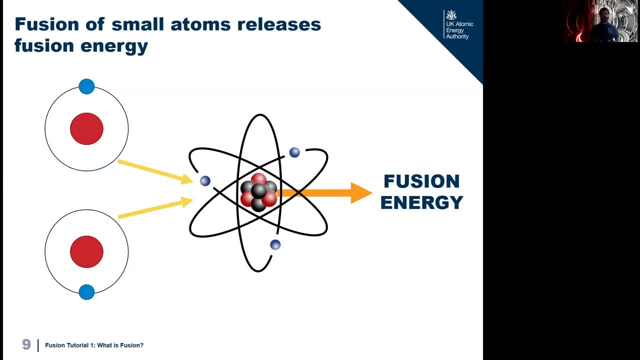 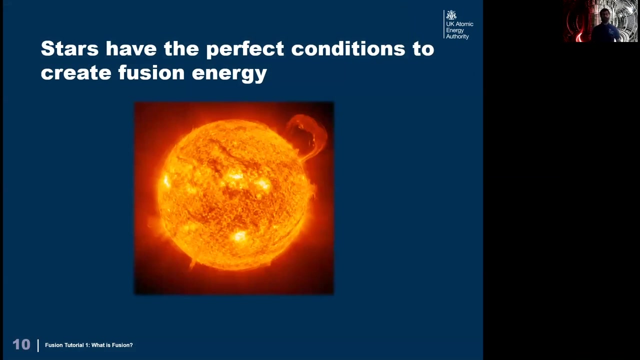 but it's actually a lot more difficult to get the conditions to force those atoms to combine and fuse. To understand the conditions that we need to release fusion energy, we need to look to the stars. Stars have the perfect conditions to create fusion energy. 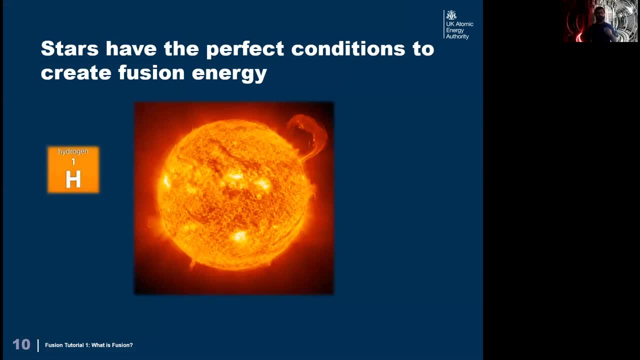 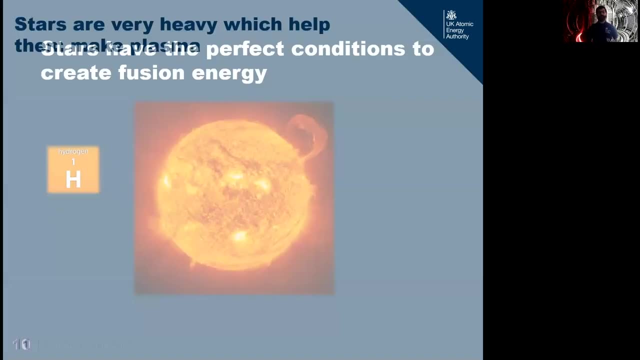 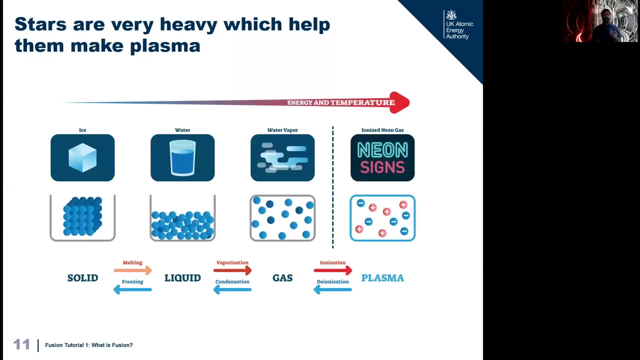 They use hydrogen-1, a basic form of hydrogen, as their main fuel, And one of the really key things for stars is that they're very heavy helping them make this thing called plasma. Now, what is plasma? Well, very simply, plasma is the fourth state of matter. 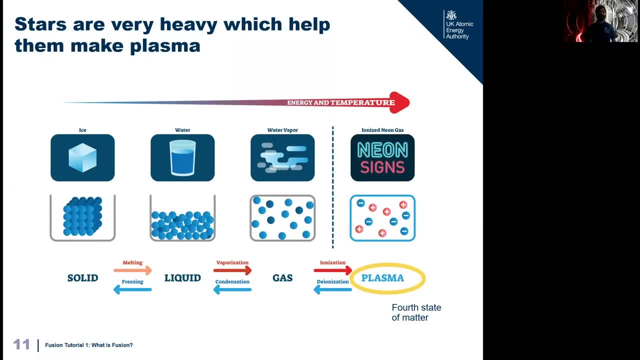 We commonly think that there are three main states of matter: solids, liquids and gas. But there is also plasma, And to achieve plasma conditions you do still need to do the same as you would for solids, liquids and gas to change between a solid liquid and gas. 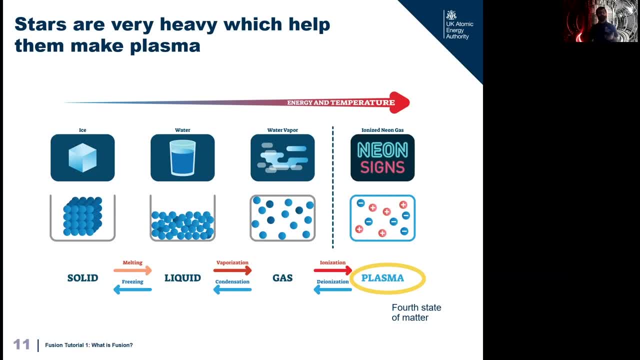 To get from a solid to a liquid, you need to heat up that solid and melt it. To get from a liquid into a gas, you need to heat up it again until it evaporates. And to get plasma, we need to superheat a gas until it ionises. 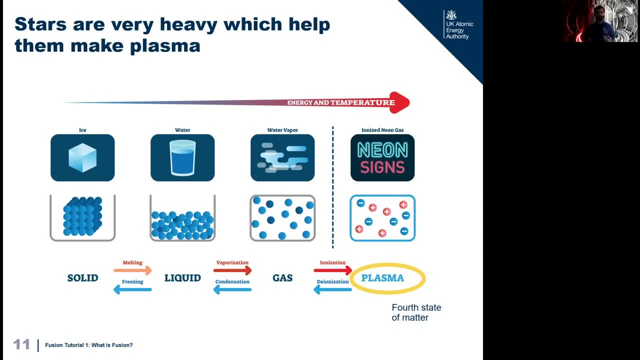 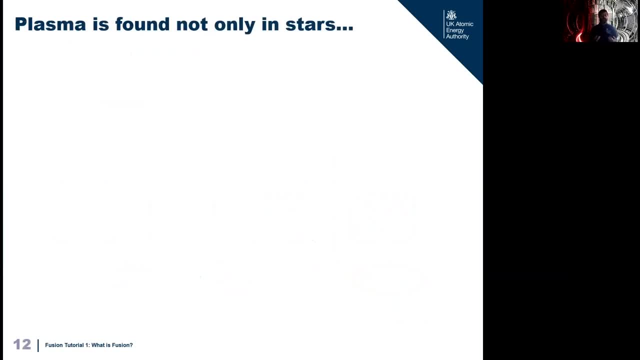 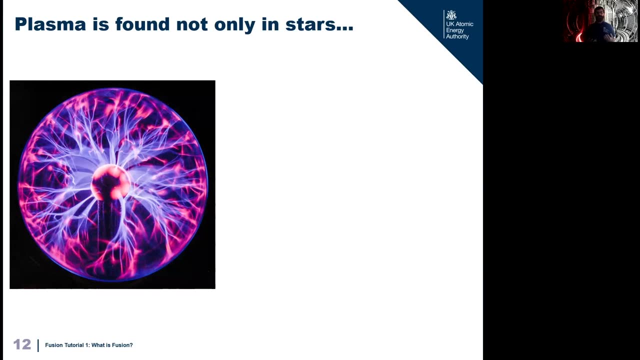 and then turns into plasma. Now, plasma is found not just in stars. This is a picture of a plasma ball. Now, if you ever come to a science festival where we're at, or if you come to one of our careers days or open days, 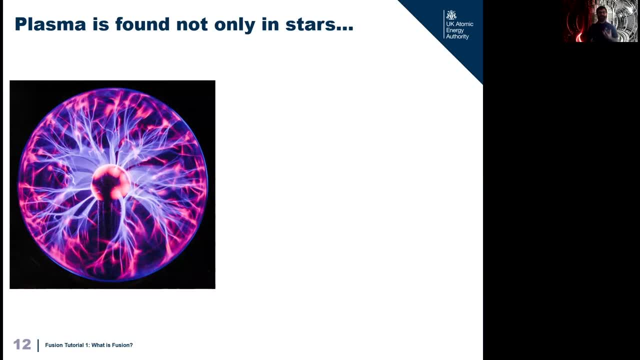 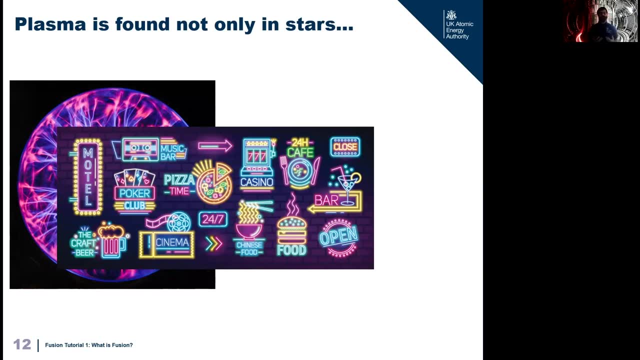 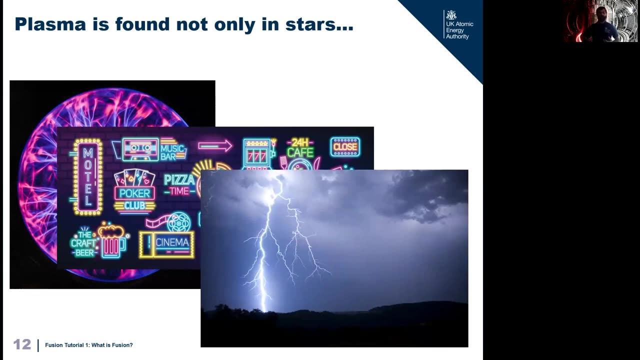 you'll be able to see plasma in action inside this glass ball. You can also see plasma inside neon signs lighting up streets, And it's the same thing that happens with lightning: When you get a big buildup of electrical charge in clouds. that electrical charge can then funnel down to Earth. 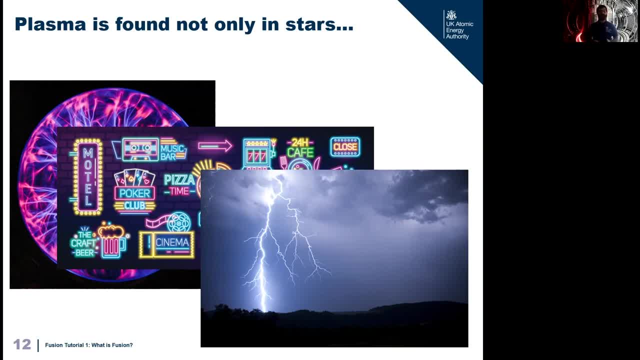 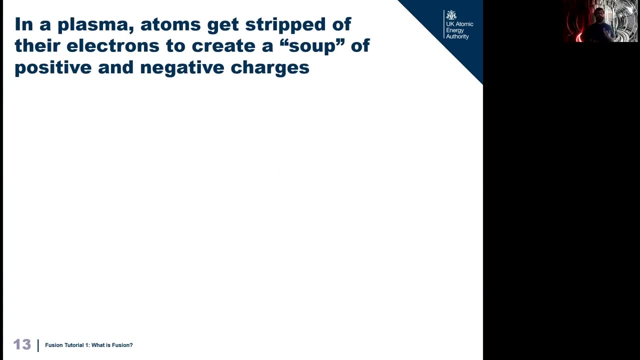 heating up the gas and the air as it comes down, ionising those gas particles in the air, turning them into plasma. Now, what actually is it like in a plasma? Well, in a plasma, atoms get stripped of their electrons, Creating a soup of positive and negative charges. 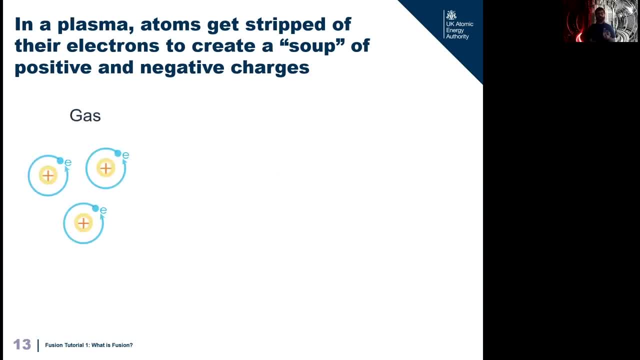 To help us understand that a little bit more, we're just going to look at a gas for first. So with a gas, this is what the atoms look like. They're very much intact. You have the electron around the outside and the nucleus in the centre. 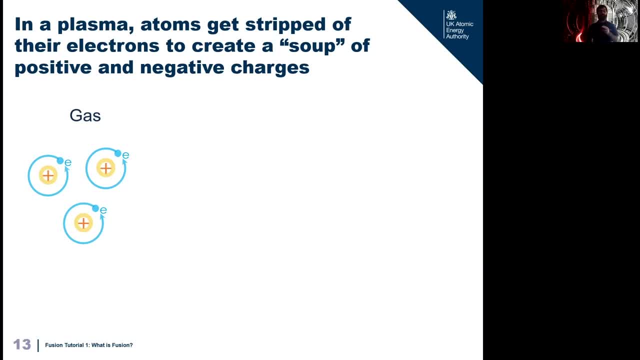 Now actually that electron is negative, So normally you would have this whirl of negative charge around the nucleus And the nucleus is positive. Now, because you have this positive and negative charge, normally in solid silicon gases, these would cancel each other out. 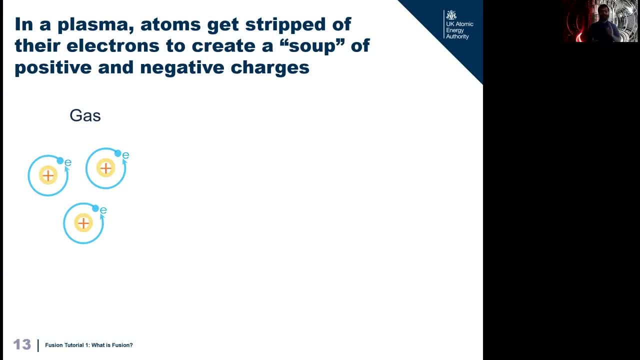 and you would get neutral atoms. But that's what's different with a plasma, Because when you superheat that gas and turn it into a plasma, the electrons get stripped away from the atom and start to move away And the positive nuclei are left. 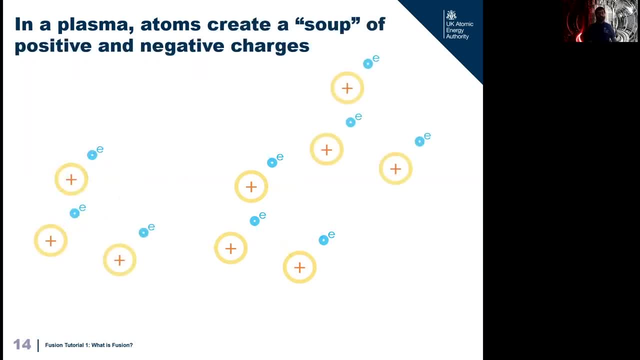 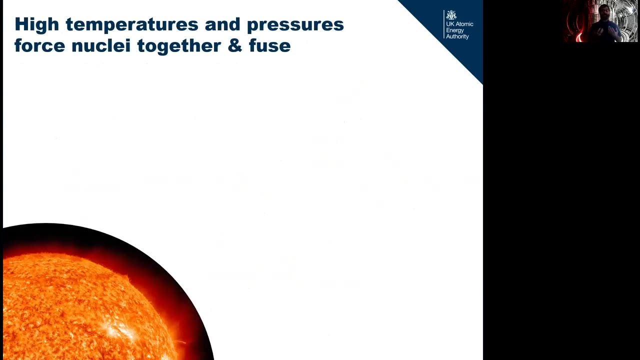 to move around by themselves And you get this soup of positive and negative charges moving around independently from each other when you have a plasma. So a plasma is key to creating the conditions of fusion, But it's not everything that you need. You also need high temperatures. 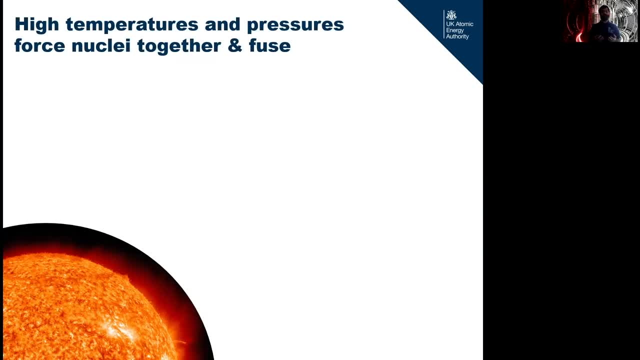 and pressures to help force nuclei together to fuse. Now inside the Sun, we get these extreme conditions. There's very high temperature, 15 million degrees in its core. There's also very high density. The particles are packed in very close and tight with each other. 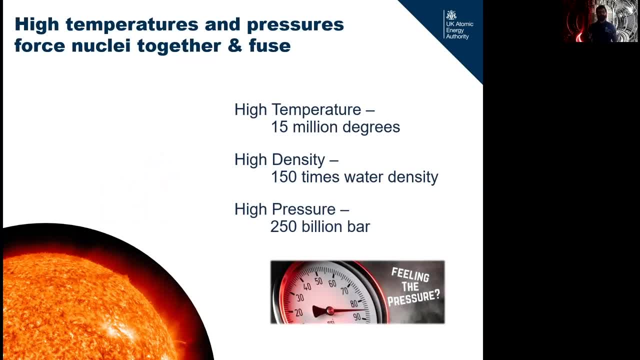 And there's also extreme pressures inside stars. 250 billion bar Sounds like a very hard number to really even understand. Well, to help myself to understand it, I looked for comparisons here on Earth And actually, if you just stand outside, 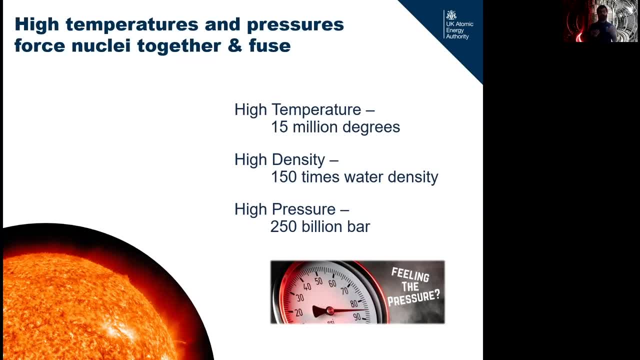 head out anywhere on the street, you'll probably experience about one atmosphere of pressure or one bar of pressure. So that's next to nothing compared to the core of the Sun. Another comparison would be if you go to the deepest part of the Earth's surface. 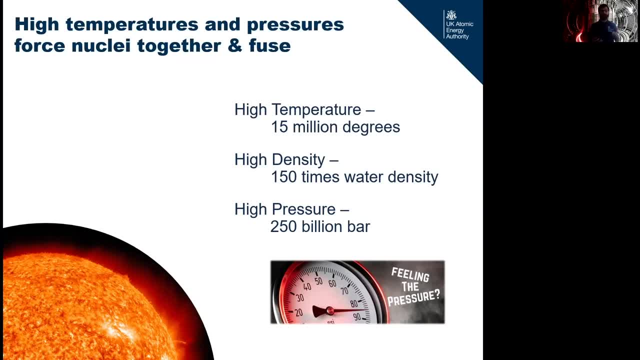 and that has the highest pressure on the surface of Earth, and that is found in Mario Trench, right at the bottom of the ocean, And there you would still only experience just over a thousand bar, In fact, if you wanted the highest pressure. 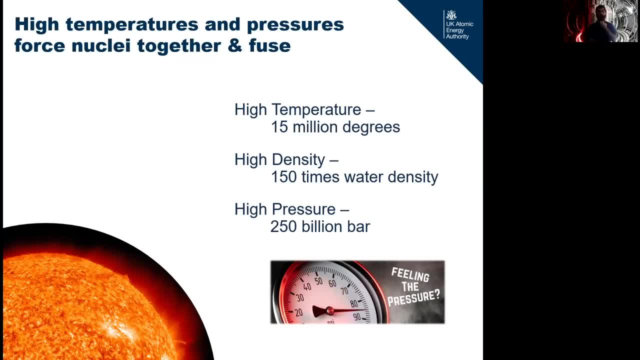 anywhere on Earth. you would have to go to the very core of our planet, And in the Earth's core you would experience three and a half million bar. That's still billions and billions away from the pressure experienced in the core of our Sun and stars. 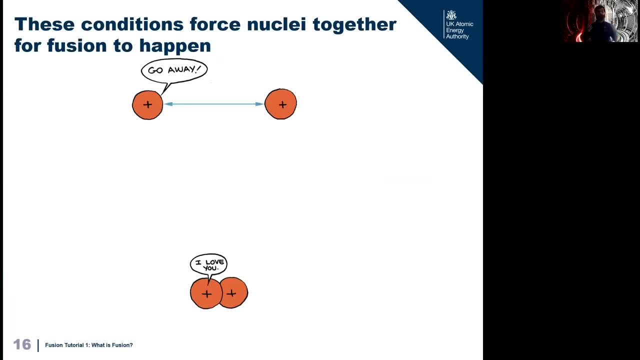 Now these conditions are what are needed to force nuclei together for fusion to actually happen, Because without these conditions you wouldn't get any fusion, You'd just have a plasma roaming around Now, if you think of a magnet and you wanted to push that magnet together, 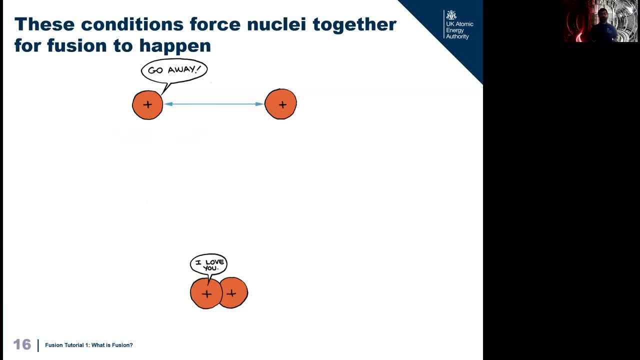 with a magnet, it would be very hard to push the same pole, say a north and north pole, together, Because naturally they would want to repel. It's the same with charged particles such as our positive nuclei, Because they're both positive. 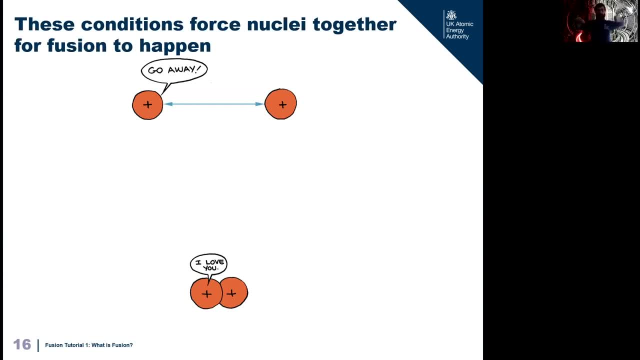 and you want to push them together, they'd naturally push apart and repel each other. It's only when you add these fusion conditions, these extreme conditions of temperature, density and pressure, that you overcome that repulsion and fuse your atoms together to release fusion energy. 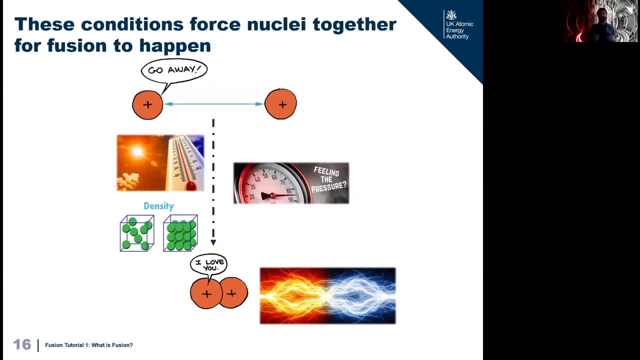 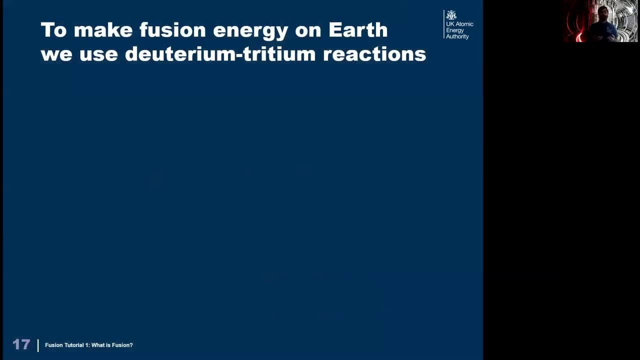 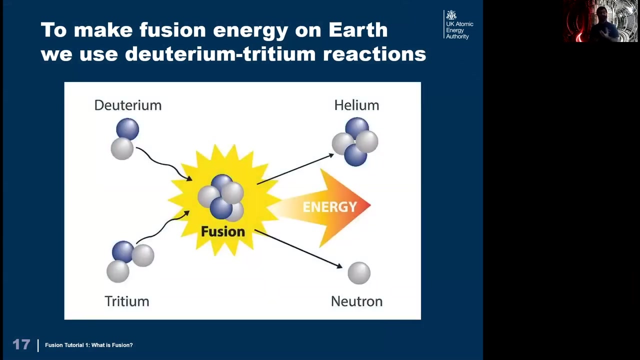 So this is how fusion happens inside stars, But we want to be able to harness that star power and recreate fusion here on Earth to power our homes. To do that, we make fusion energy on Earth using deuterium-tritium reactions, And this is the specific reaction. 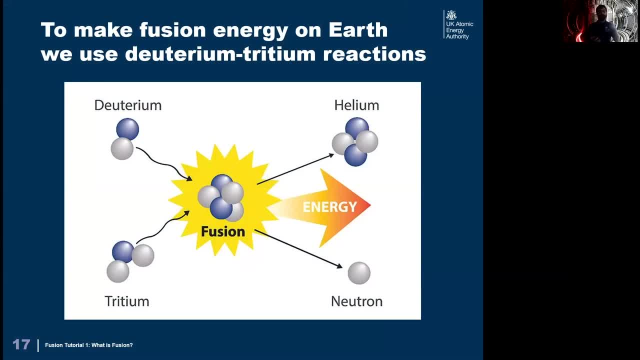 that we work on here. We get deuterium and tritium, those heavy isotopes of hydrogen force them together, make fusion happen, which then releases helium, neutrons and energy, And we're going to have a little bit more. 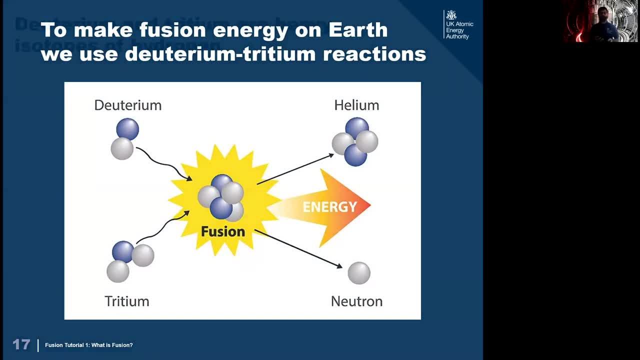 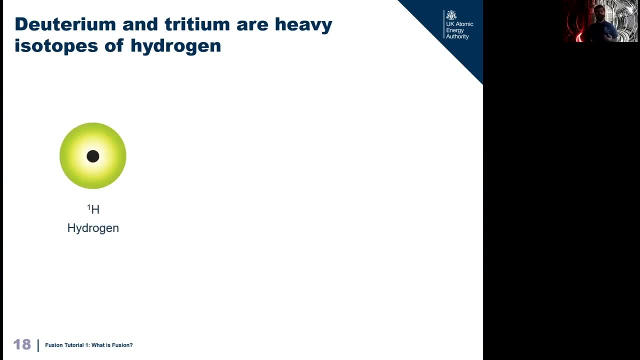 of a look at this reaction shortly, But just as a little reminder, remember that deuterium and tritium are just heavy isotopes of hydrogen, So basic hydrogen hydrogen-1 will just have a proton. deuterium has a proton and a neutron. 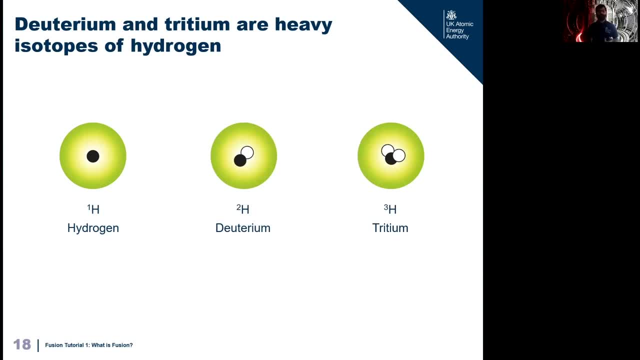 and tritium has a proton and two neutrons, giving us hydrogen-2 or deuterium or hydrogen-3 or tritium. Now these two reactions, or these two isotopes, when they're reacted together, are actually the most efficient. 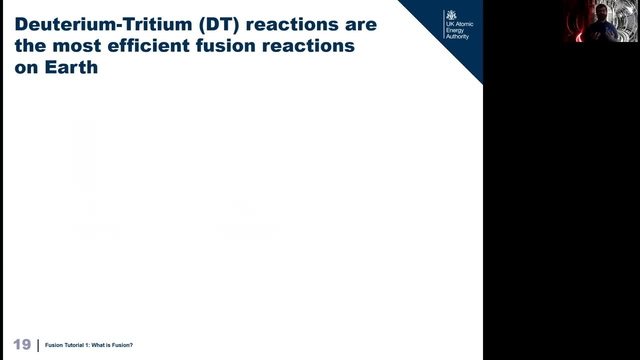 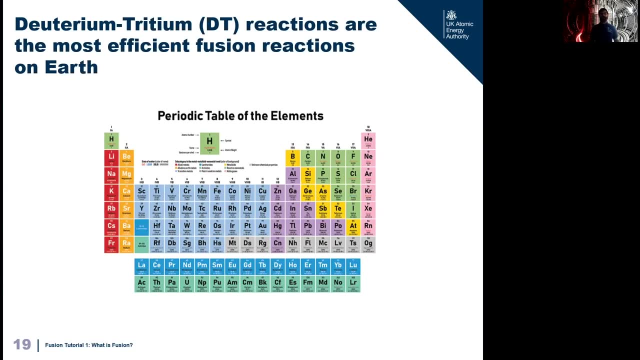 fusion reactions on Earth, And that's fundamentally why we use deuterium and tritium. You might think that we could use any element in an empiric table. Well, actually, firstly, not all elements are able to fuse And secondly, 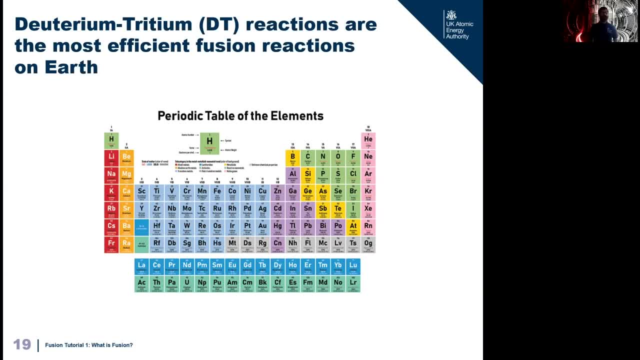 as you get higher and heavier with the atoms you're getting less efficient. So hydrogen itself is a very efficient way of producing fusion, And deuterium and tritium are isotopes, are heavier isotopes of that hydrogen. Now I mentioned that stars use hydrogen. 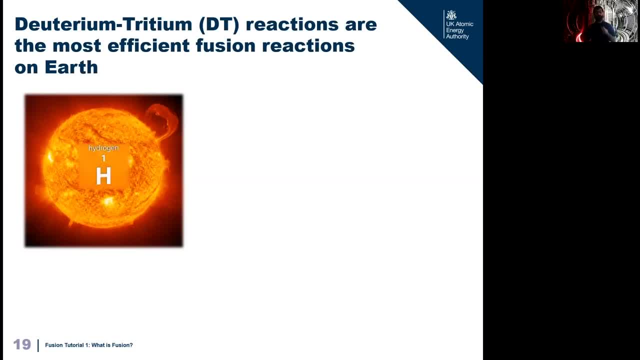 Mostly they run off hydrogen-1 as their core fusion fuel, And when you fuse hydrogen together you create helium, just like with the reaction we're trying to create here on Earth, But then you can actually keep on fusing other elements, So you can fuse helium. 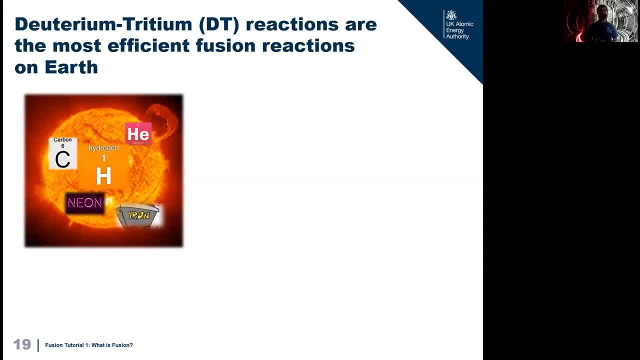 which will then fuse into other things, and then eventually you'll get carbon, neon and ultimately iron. Iron is the most stable atom and therefore one of the ones that you can't really fuse any further. There are special ways of fusing heavier elements together. 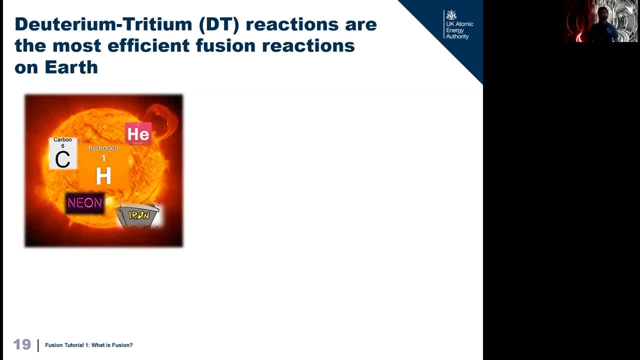 in celestial events such as supernovae, that can create all the other elements in the periodic table, But inside stars you're fundamentally just getting hydrogen as the core fusion fuel. Now, with our Sun, our Sun's lifespan, with hydrogen fuel, 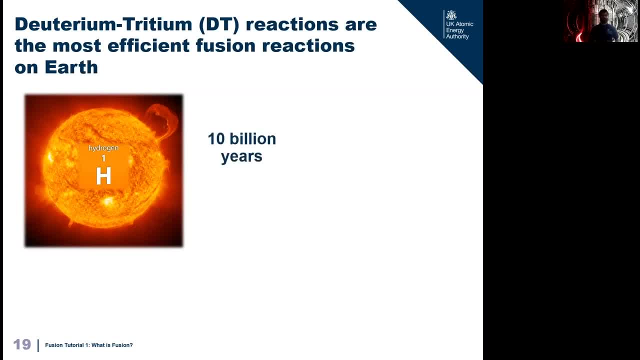 is going to last about 10 billion years. It's a really really long time in our kind of light thinking, But our Sun is already about halfway through that life cycle. It's about 4.5 billion years old, So it's got a good another 5 billion to go. 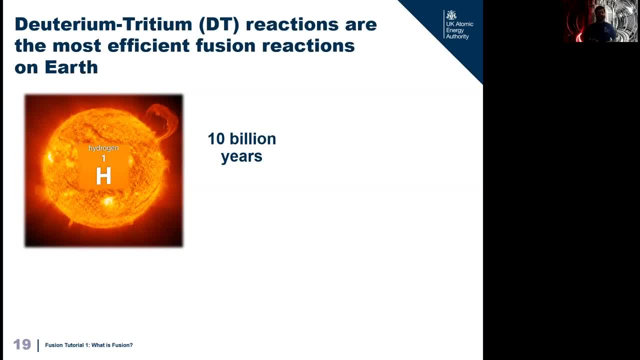 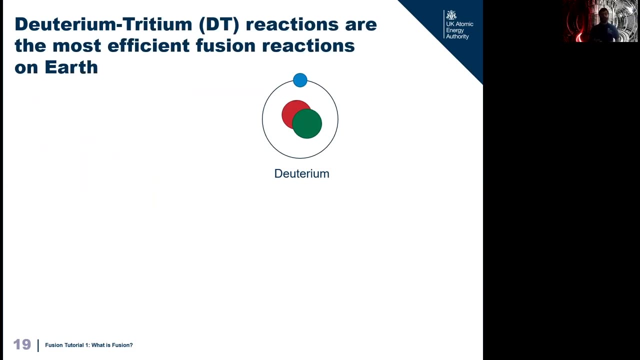 But if it was made of deuterium, that wouldn't be the same story. So if the Sun ran on deuterium fuel instead of hydrogen one, it would have gone in a flash lasting only a few seconds or less, instead of that 10 billion years. 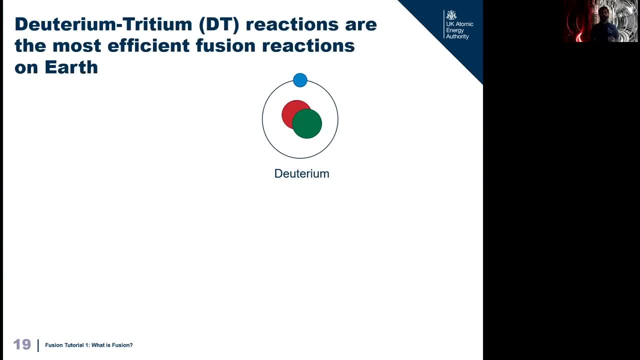 that our current Sun will run with hydrogen one. Now, when we combine deuterium with a super heavy hydrogen tritium, we get even more efficient fusion reactions, And this is why we use them. We use these heavy fuels so that we can compensate. 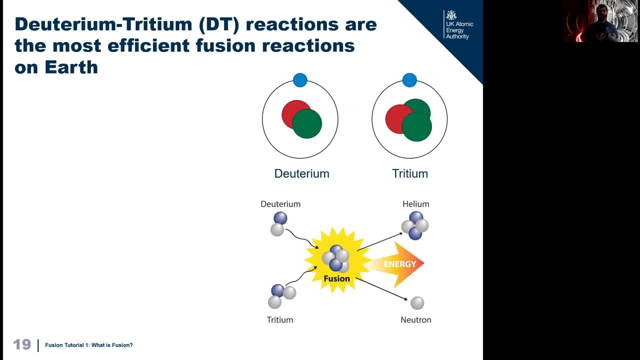 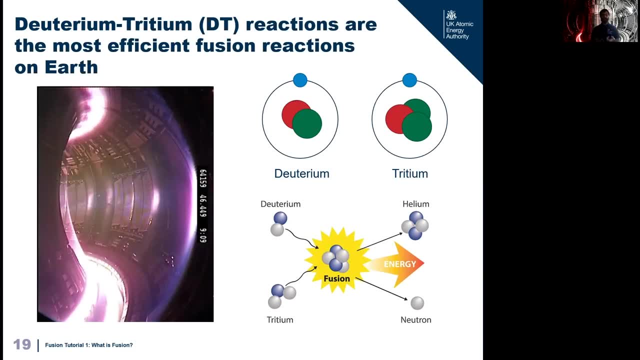 for the extreme conditions experienced in the Sun and recreate fusion here on Earth. And this is a picture of fusion happening inside one of our machines. The machine is called JET or the Joint European Taurus, And at UK we're very lucky to be able to host and operate JET. 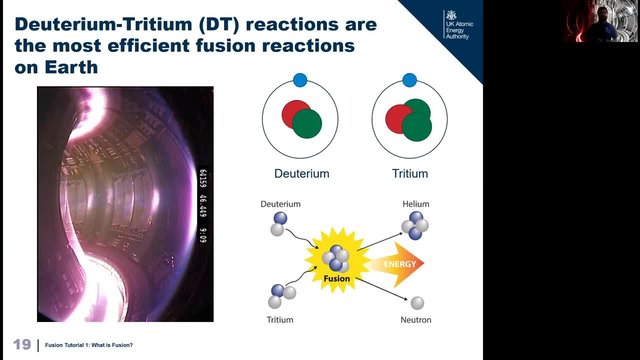 on behalf of the Eurofusion program. And JET is the largest fusion tokamak in the world, The only one currently capable of using a tritium fuel. Now that's really important because this means that we can run experiments that will look like the real fusion fuel. 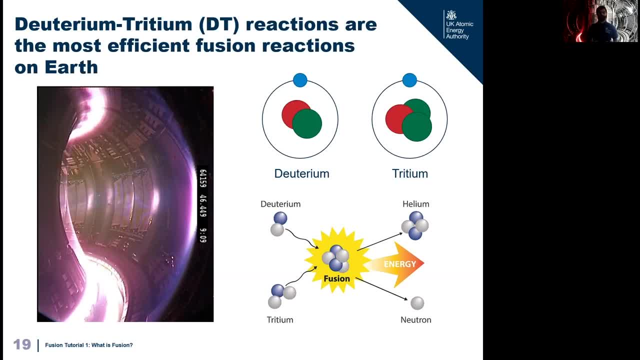 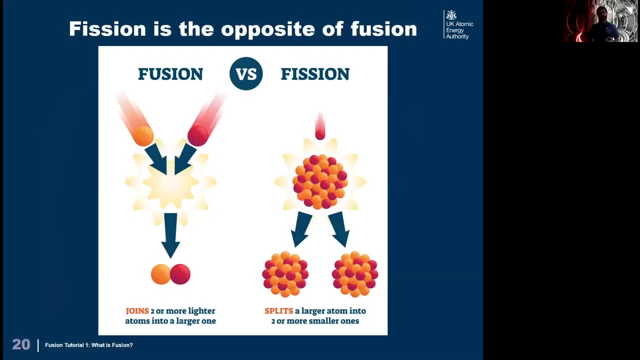 we're going to be needing for fusion power stations in the future. So this is how we are trying to recreate fusion here on Earth. But that's not the whole story. Now I wanted us to talk about fission, because fission is the opposite of fusion. 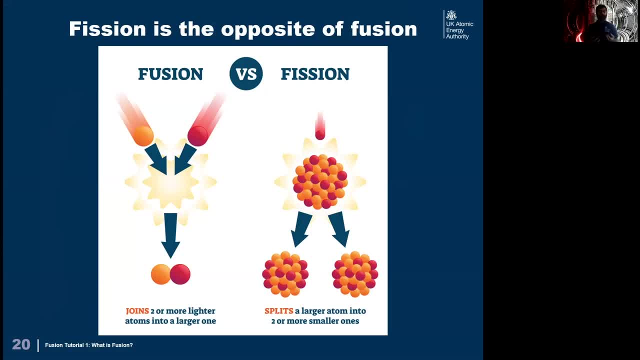 Now, fusion, as we now know, is what happens when you take small light atoms and fuse them together and then energy was released that way, Fission being the opposite, is what happens when you take big heavy atoms and they split up and you also get energy out at the same time. 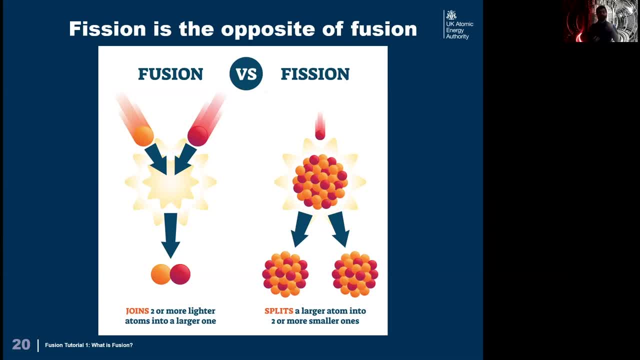 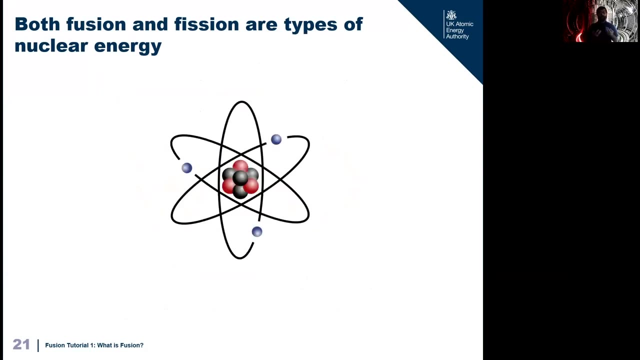 Now, the reason why we're bringing up fission is because this is the current type of nuclear power that we have, providing energy onto the national grids, And that is because both fusion and fission are types of nuclear energy And all nuclear energy means. 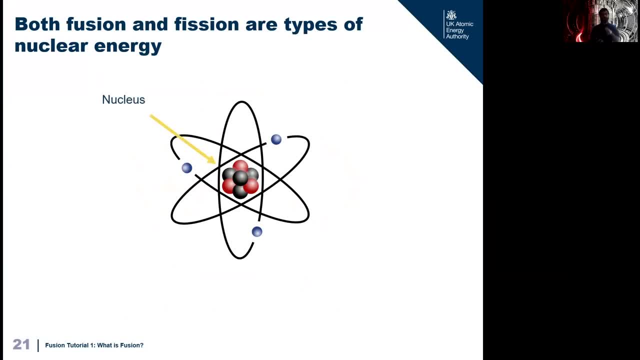 is that we can get energy out of the nucleus of atoms in nuclear reactions. Now, the two types of nuclear reactions that we've got here are fusion, where you're taking those small atoms and combining them together to get fusion energy, or you take larger, heavy atoms. 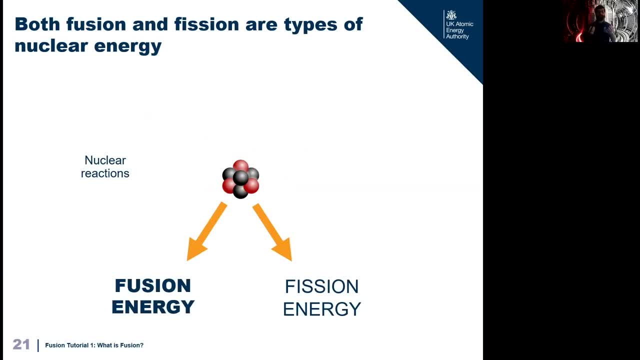 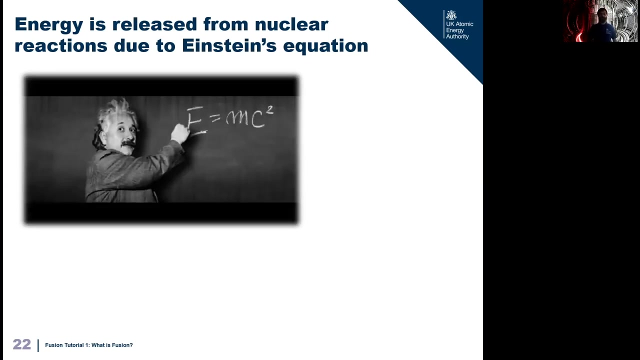 and split them up or fiss those nuclei to release energy. How do we know that we can get enough energy from these reactions to be able to one day power power stations? Well, it's all thanks to Einstein and probably the most famous equation in science. 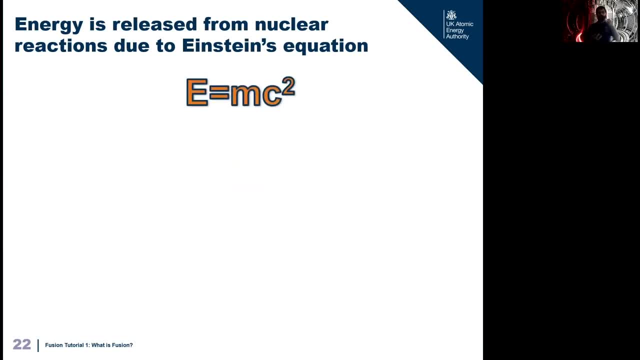 E equals mc, squared Now. that stands for energy equals mass times, c, which is this constant, the speed of light, squared Now, because c is a constant, you can almost forget about it and think of this equation as a relationship between energy and mass. 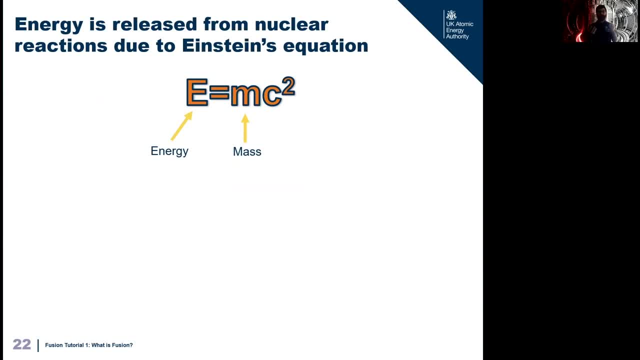 And because these two things are related, whenever there's a change in one or the other, whenever there's a change in the reaction, you get a change in the other side. So how does this look with our reaction? Well, our reaction is deuterium plus tritium. 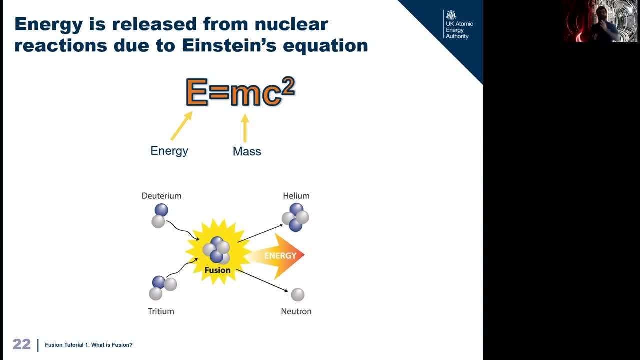 fused together and then release out energy at the same time as helium and a neutron. Now in this system the mass is rearranged because, even though taken together, the helium and neutron have the same total number of protons and neutrons compared to deuterium and tritium. 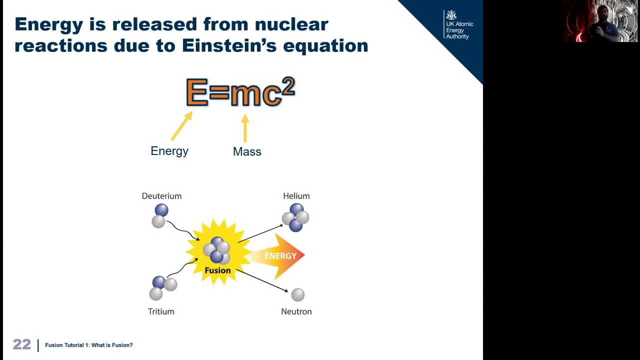 that goes into the reaction. the protons and neutrons are arranged differently in the helium and neutron And that different arrangement causes a release of energy because there's been a change in the E equals mc squared equation in the relationship. Now fission reactions. 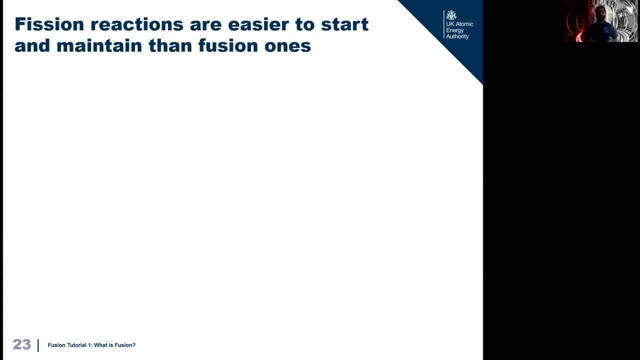 can also get energy, just like our fusion one, And in fact they are much easier to make happen and to maintain and keep happening than fusion reactions. So here is a nuclear power station we might have at the moment and it uses this series of fission reactions. 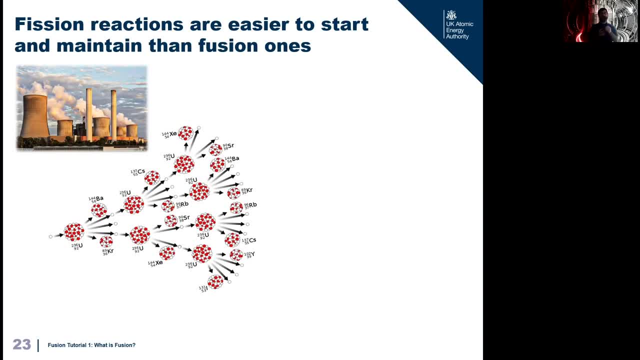 We take a very big heavy atom and then split it up, and then it starts to hit other heavy atoms which then split up, and then those split up and split up and you end up with a chain reaction happening. Now this means that the reaction can just keep on going. 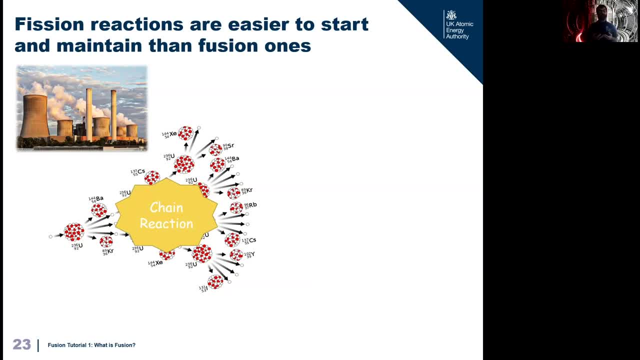 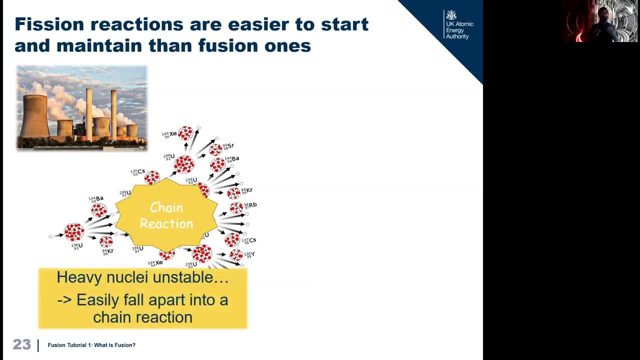 Now, why does the chain reaction happen in the first place? Well, heavy nuclei are actually very unstable, and unstable nuclei easily fall apart into these chain reactions. But this isn't the case with fusion at all. Remember, fusion is the opposite. So we have to start off. 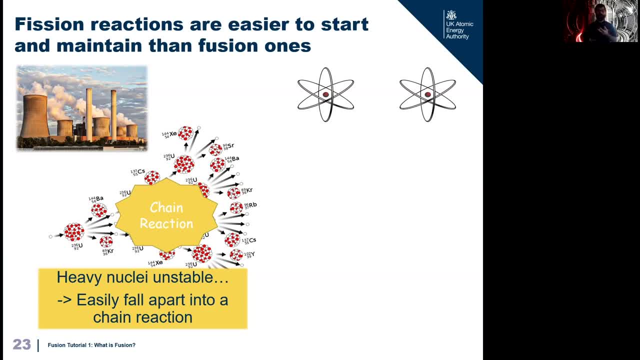 with small light nuclei when we're using fusion, and then they combine together, creating heavier atoms. Now, because we're starting with small light nuclei, those are actually very, very stable and they don't often want to change or fuse together To make them have to fuse. 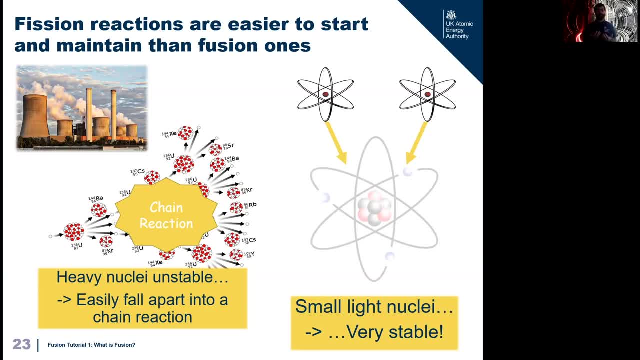 we have to continually produce these extreme fusion conditions, And what that means is that we're not getting a chain reaction and we're always having to put in effort to produce fusion energy with a fusion reactor. So achieving conditions for fusion is very, very difficult. 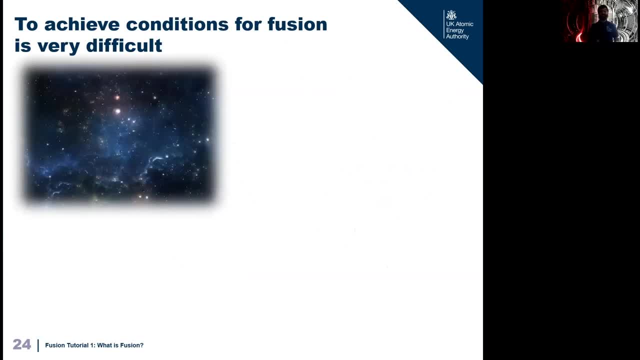 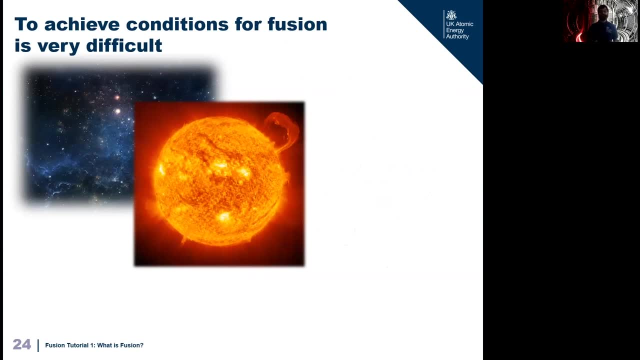 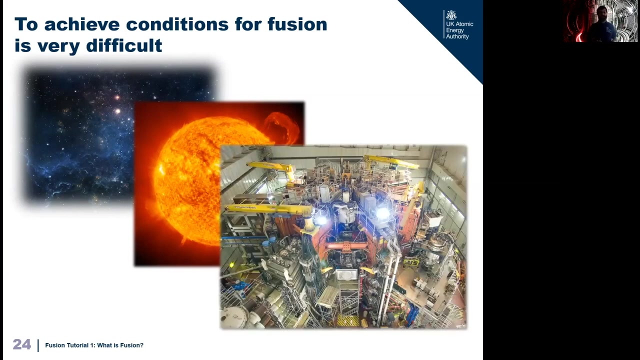 So difficult because we're trying to recreate stars. We're trying to recreate the reaction that powers our Sun, that gives off enormous heat and light, travelling through space where we feel here on Earth and see. Now this is our fusion machine, is JET. 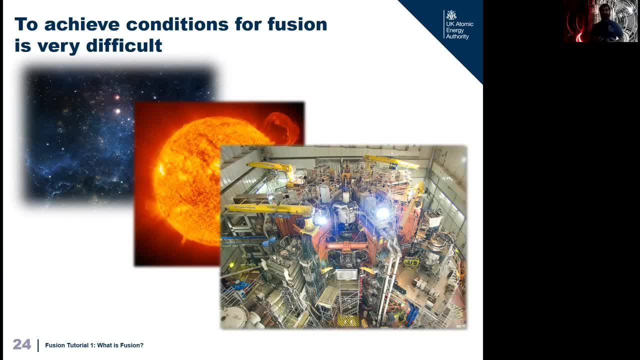 You can see that it's a very complex machine. There's lots and lots of engineering that goes into this project and we get lots of science out. Now this machine is still an experimental machine and that's why we're still understanding the science and getting so much scientific research done. 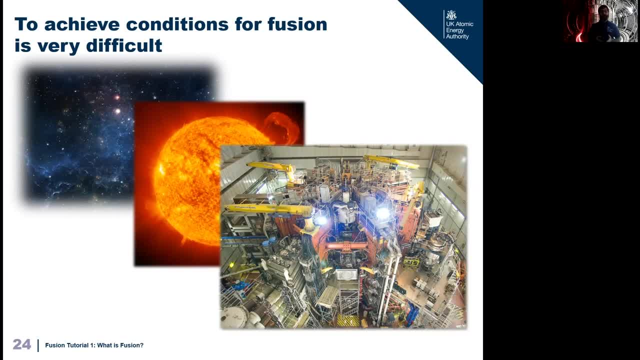 with JET. The next step is going to be taking all of the knowledge that we've understood from JET and using those engineering skills to build power stations that run on fusion energy. So we've made fusion happen and we're now taking it to the next step. 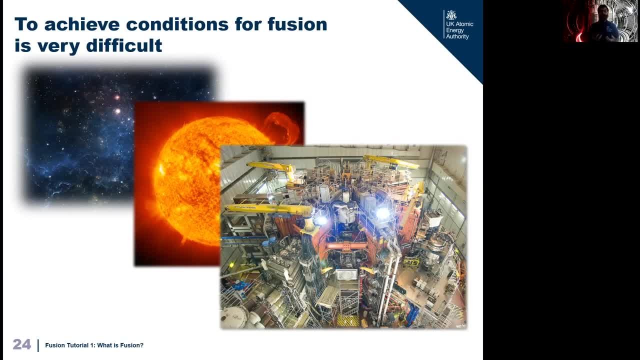 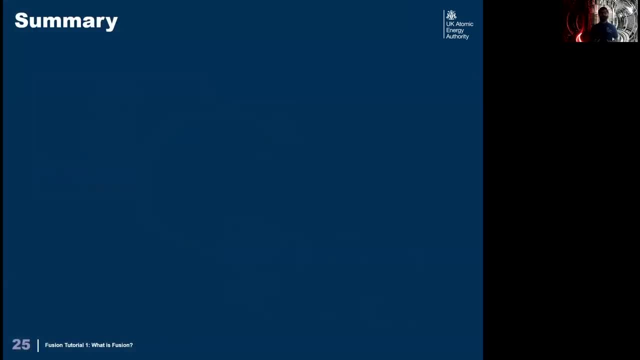 to try and bring fusion energy out as a power source that we can use to power our homes. And that brings me towards the end of the first fusion tutorial. So just to have a little bit of a recap and a look at what we've covered, 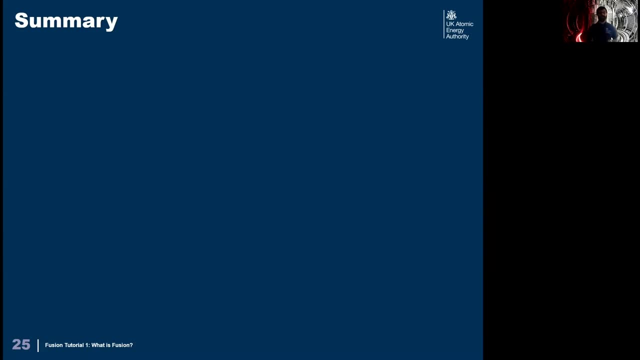 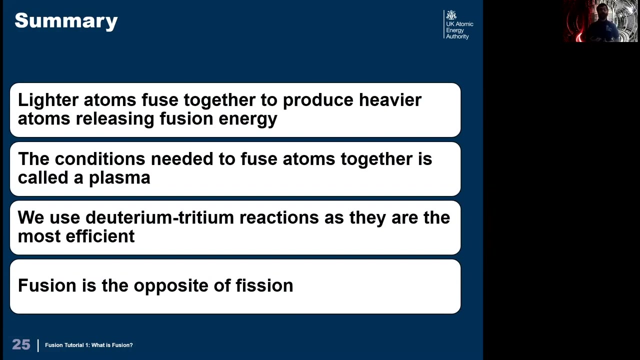 we've answered those first four questions we had at the start of this. The first one was: what is fusion? And the answer was that lighter atoms can combine or fuse together to produce heavier atoms and release fusion energy. And we looked at the conditions of fusion.